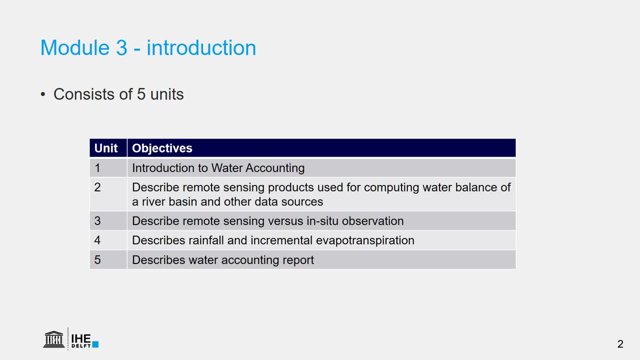 Unit 2 is devoted to describing remote sensing products used for computing water balance of a riverbed and other water resources. Unit 3 discusses how we can compare remote sensing data with in-situ observations and infer reliability of remote sensing data used for water accounting. 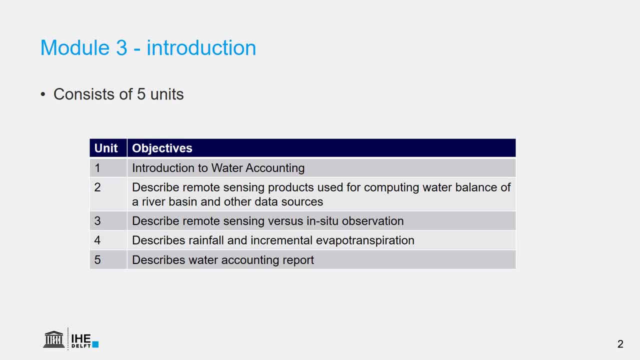 It also shows how to perform precipitation and evapotranspiration computation per land use or land cover classification. Unit 4 is about rainfall and incremental evapotranspiration. It describes rainfall incremental evapotranspiration. It describes the need to split evapotranspiration to its rainfall incremental components. 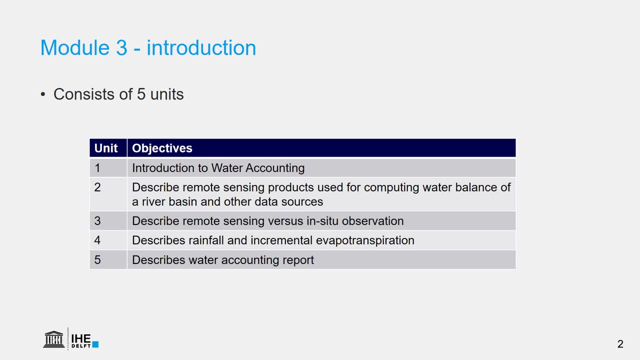 It also discusses the various meters used to split evapotranspiration. It provides an exercise where we use a soil-moisture-water balance model to split evapotranspiration. The last unit- Unit 5, describes water accounting. It mainly discusses the resource base sheet and the accompanying tables and the maps of. 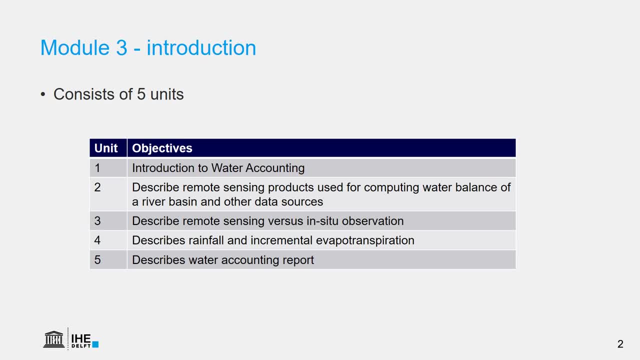 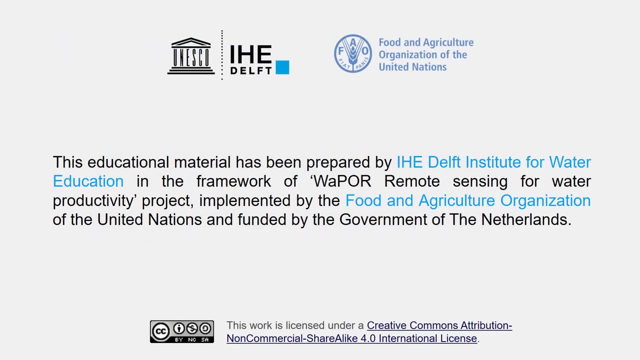 the water accounting report. It also discusses key indicators of the state of water resources in river basin. This educational material has been prepared by IHE Delft Institute for Water Education in the framework of VAPOR remote sensing for water productivity project implemented by. 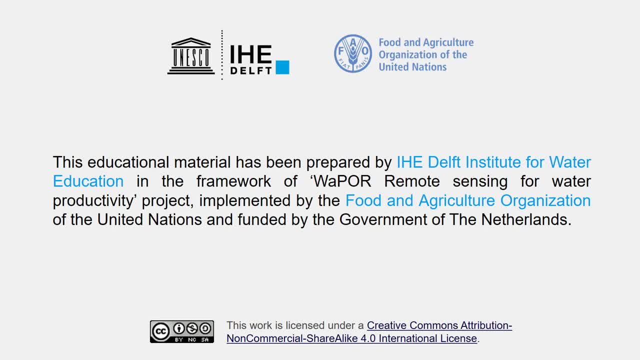 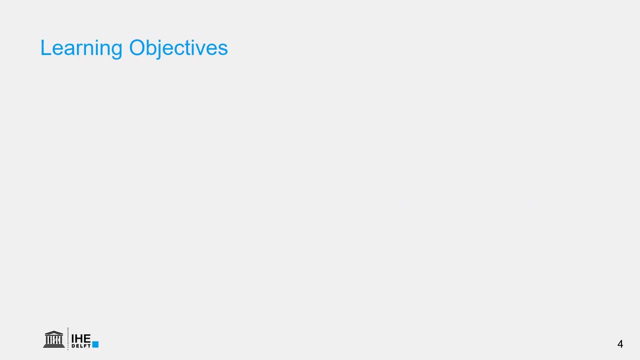 the Food and Agricultural Organization of the United Nations and funded by the government of the Netherlands. In this video, we will start the first unit of module 3.. After completing the first unit of this module, You will be able to describe what we mean by water accounting. 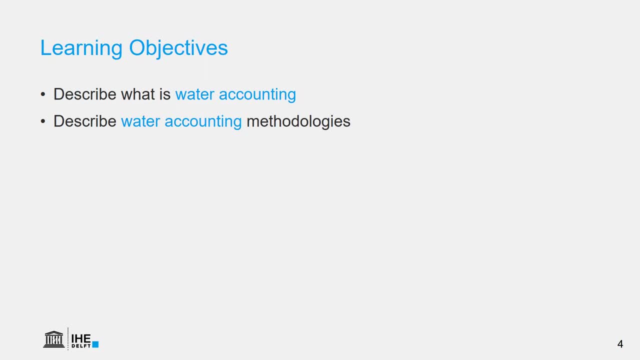 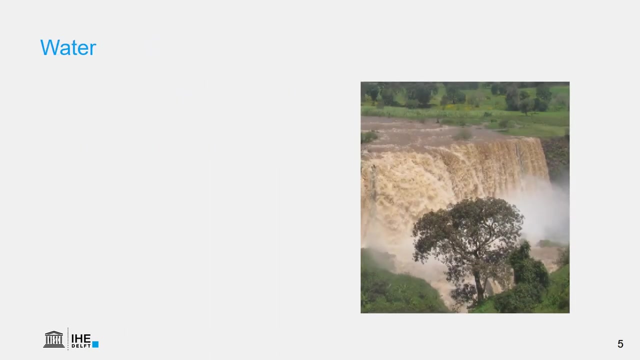 Describe some of the methodologies used to perform water accounting of a river basin, and also you will be able to describe the relevance of water accounting to integrated water resources management. Water is a unique resource. Everything in the planet depends on water. Water is a unique resource. 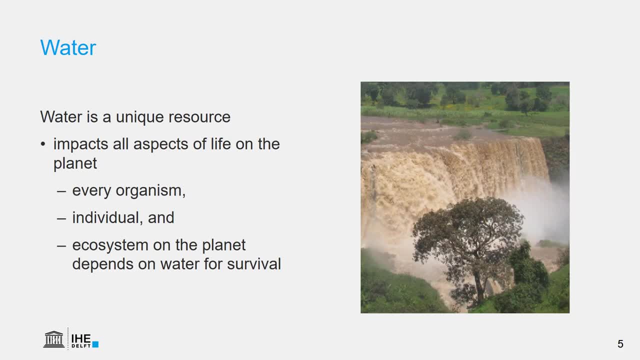 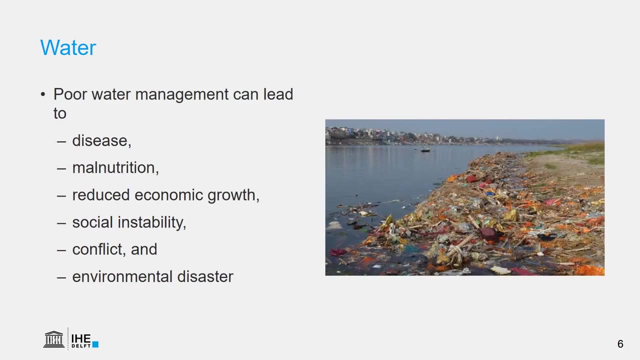 Water for survival. Every organism, every individual and ecosystem on the planet depends on it. Water impacts all aspects of life on this planet, Because water impacts everything. If water is managed poorly and its shortage can lead to stress consequences, It can lead to diseases and malnutrition. 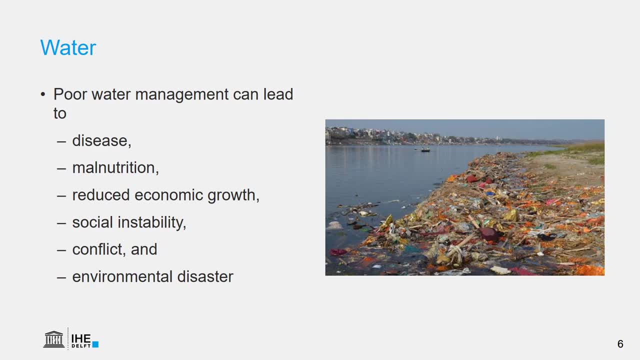 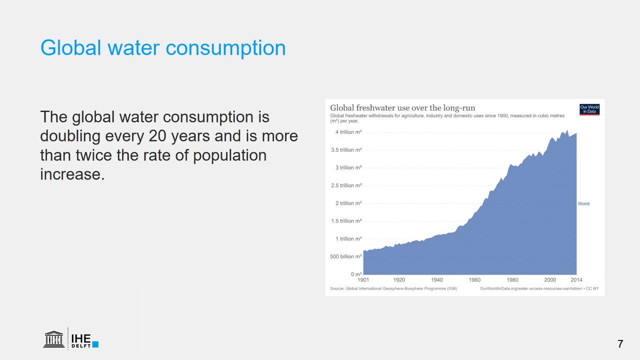 Economic growth can be affected. It can lead to social instability and conflicts. The environment will be negatively affected because of poor water management and water shortage. When we look at the global water consumption, it's doubling roughly every 20 years, More than twice the rate of population growth. 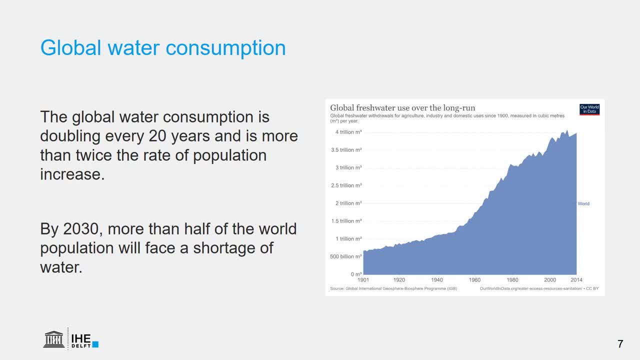 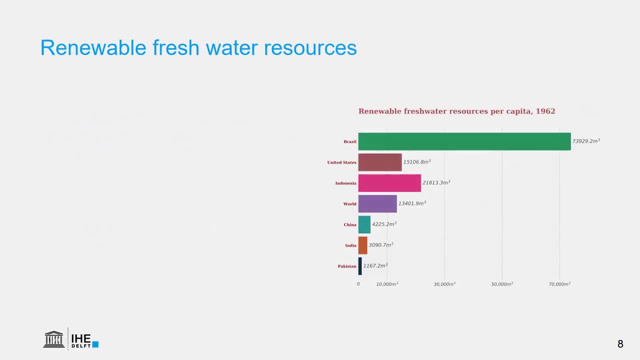 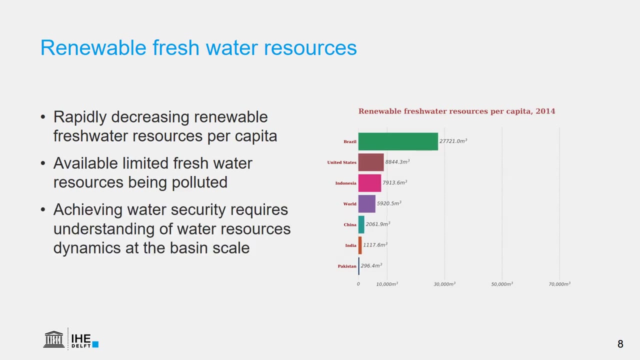 The forecast is already in progress. The population is growing. In 2030, more than half of the world's population is going to face water shortage. Availability of renewable freshwater resources per capita is decreasing very rapidly. This limited freshwater resources are becoming more and more polluted. therefore, achieving 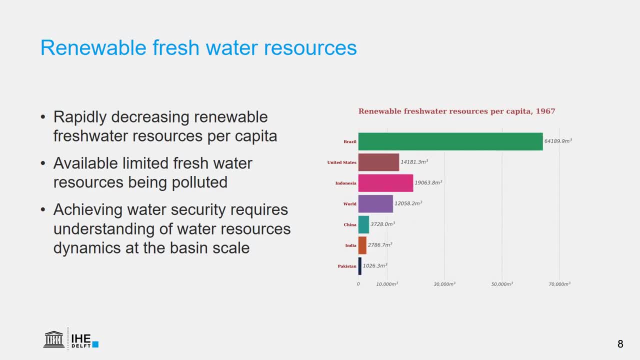 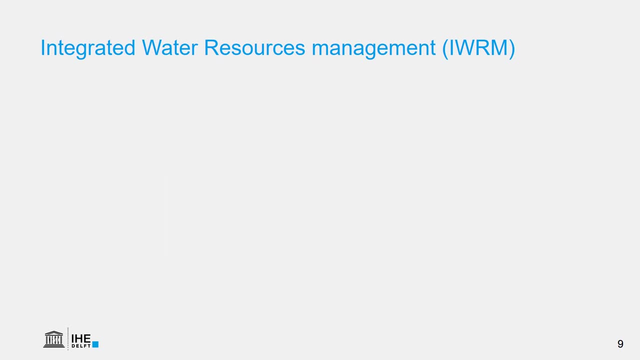 water security And increasing water quality And increased resilience to hydrological extremes requires a good understanding of water resource dynamics at the business scale. Integrated water resource management calls for sustainable management of water resources to ensure that there is enough water for future generations And that the water meets high quality standards. 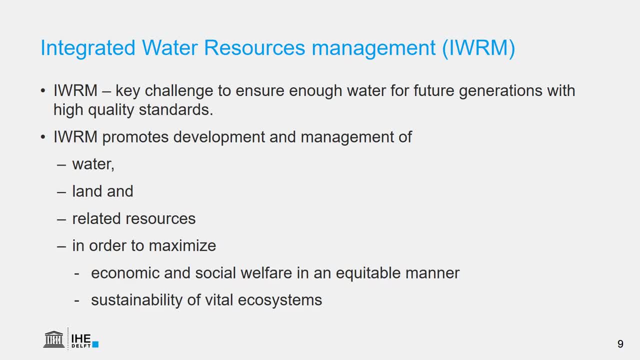 An integrated water resource management approach promotes the coordinated development and management of water, land and related resources in order to maximize the resultant economic and social welfare in an equitable manner, without compromising the sustainability of vital ecosystems. Thank you, Thank you, Thank you. 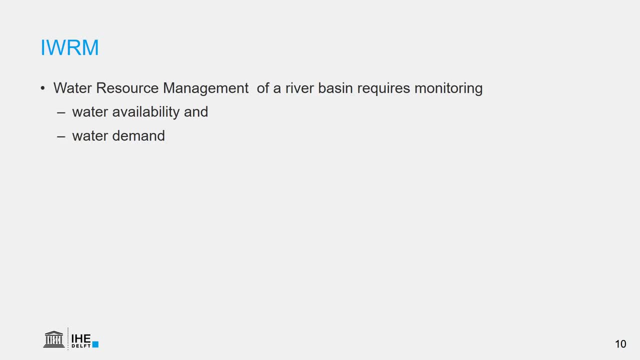 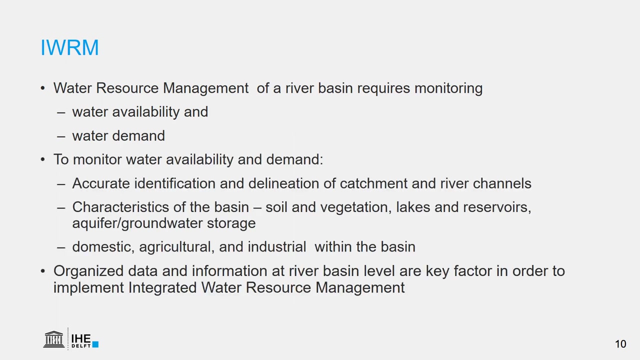 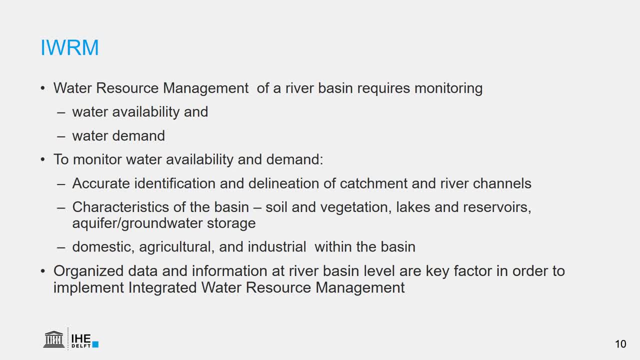 Integrated water resource management requires accurate identification and delineation of catchment in the river channels With abysmal water within a basin based on terrain and slope. It requires characteristics of the basin, such as soil, vegetation, lakes and reservoirs. 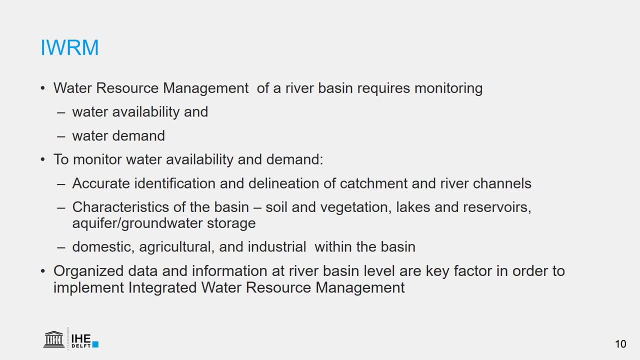 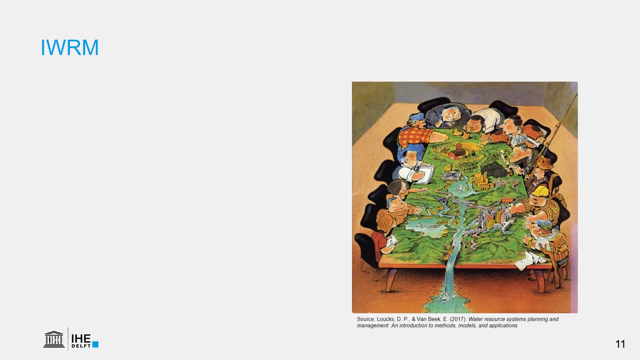 and groundwater storage. It also requires information about water demand, domestic demand, agricultural demand and industrial demand within the basin. Therefore, organized data and information at river basin level are key factors in order to implement integrated water resources management. Increased stakeholders involvement in water management. 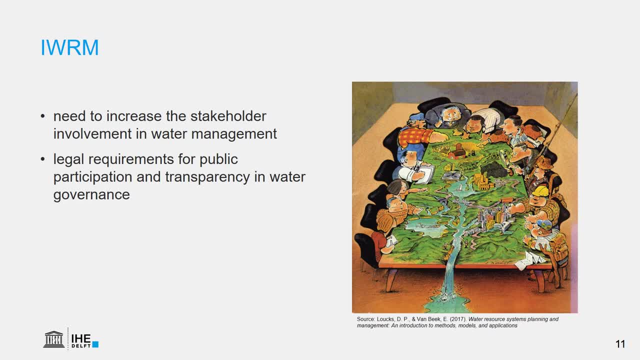 is vital for implementation of integrated water resources management. This need has been translated into legal requirements for public participation and transparency in water governance. The implementation of those legal requirements calls for making information about water publicly available in a clear and accessible way. Water accounting emerges as a useful tool. 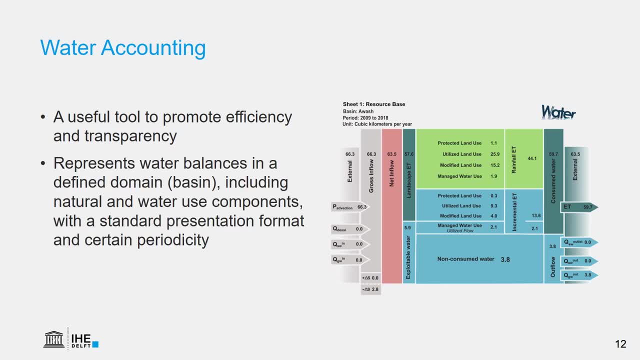 to promote efficiency and transparency. Water accounting represents a way of compiling water balances in a defined domain, including different water use components, With a standard presentation format in the water management. the gesamte softwares is built in these brains. Water accounting represents a way of compiling water balances in the defined domains, including different water use components, with a standard presentation format in the water management. 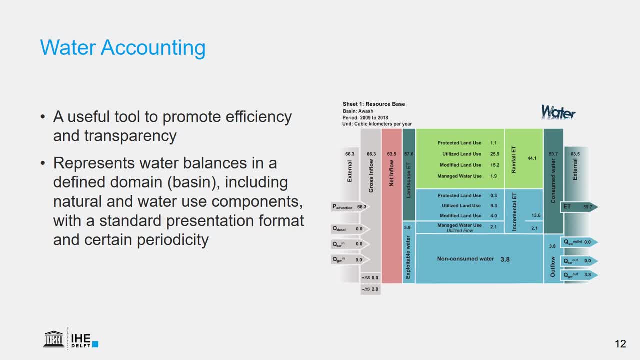 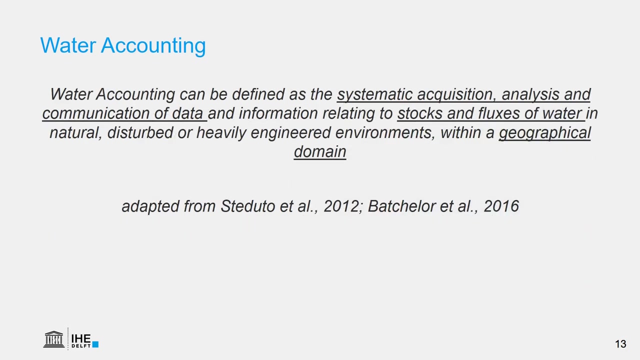 form of standardized sheets, maps, figures and tables in a defined time step. The domain can be an irrigation scheme, a river basin, an industrial region or a country, and the time step can be monthly, seasonal or yearly. A more formal definition of water accounting is adopted from literature as the systemic 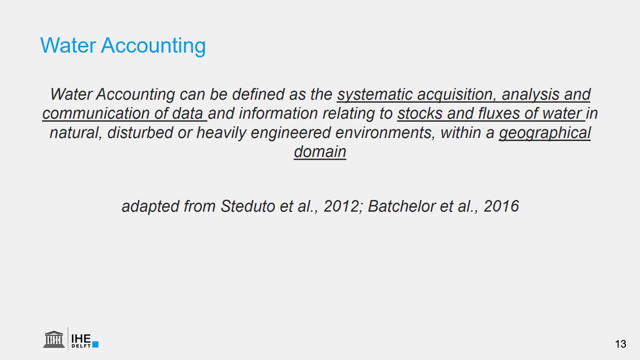 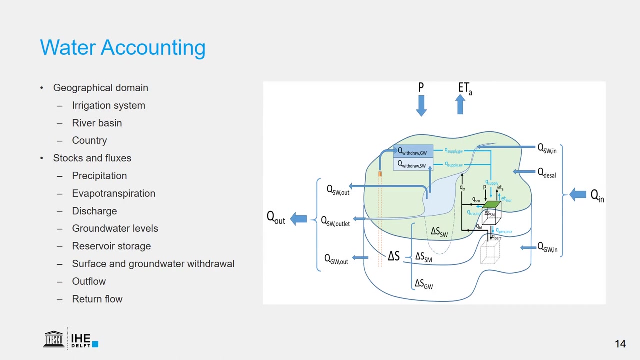 acquisition, analysis and communication of data and information related to stocks and fluxes of water in natural, disturbed or heavily engineered environments within a geographic domain. Geographic domain can be as small as an irrigation scheme or a river basin and any administrative region, including countries. 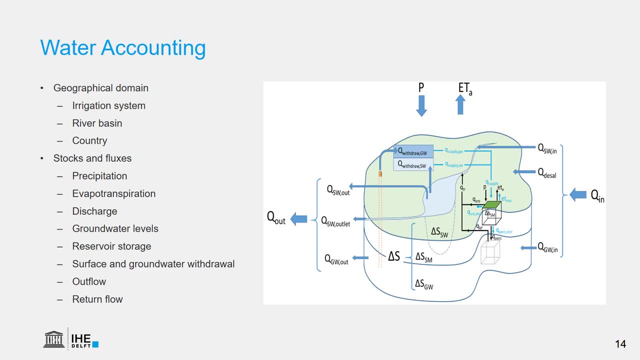 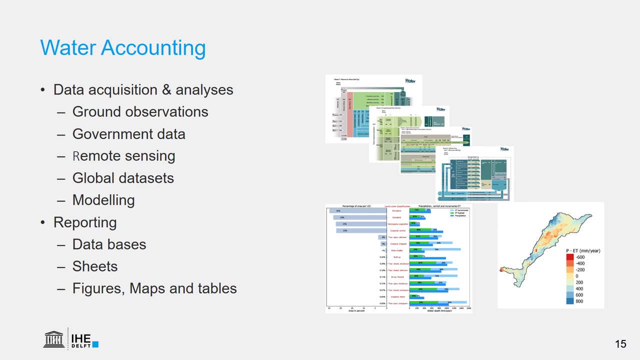 Flexes and stocks include precipitation, evapotranspiration and flows and storage. The data can be collected from different governmental organizations: ground observations, remote sensing and modeling results. The results are presented in different formats, including databases, standardized sheets. 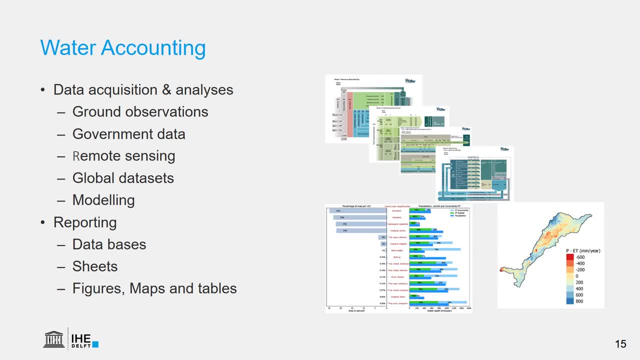 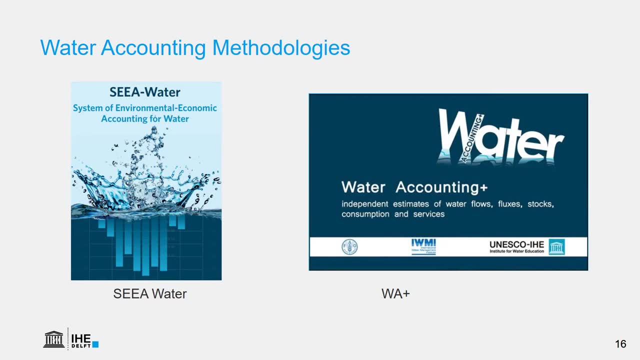 maps, figures and tables. The results can be taken from a database standardized sheets, maps, figures and tables. The results can be taken from a database: standardized sheets, maps, figures and tables. There are various water accounting methodologies in use. however, we are going to discuss here. 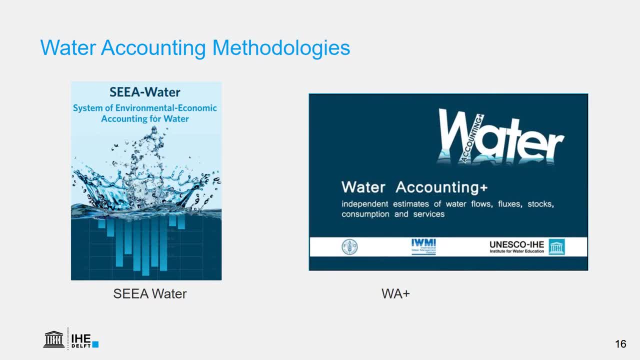 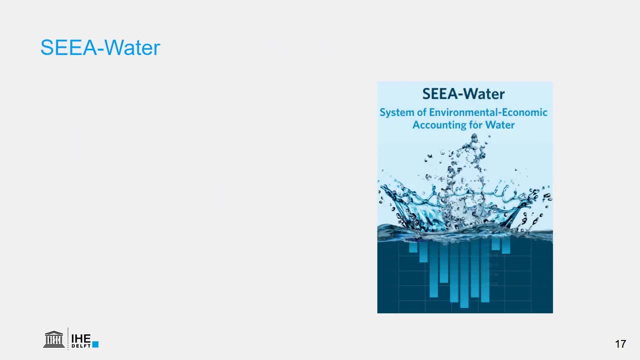 only two of the methodologies, which are the System of Environmental Economic Accounting for Water, or CEA Water and Water Accounting Plus. The first example of standardized water accounting was developed in France in the early 80s. Its purpose was understanding the impact of water use and management on the economic sector. 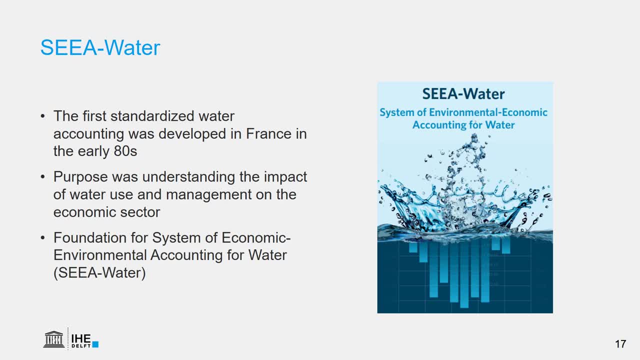 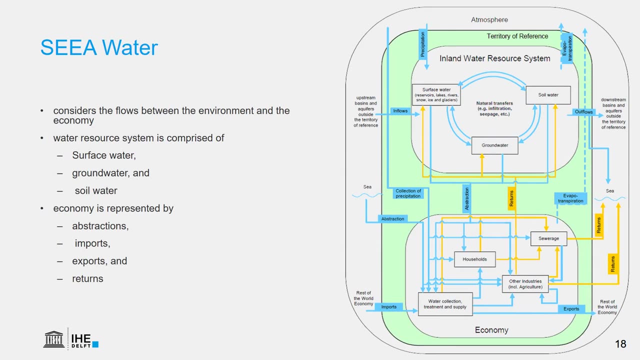 This concept was the foundation for the development of the System of Economic Environmental Accounting for Water- CEA Water. The CEA Water Framework considers the flows between the environment and the economy. The inland water resources system is comprised of surface water, groundwater and soil water. 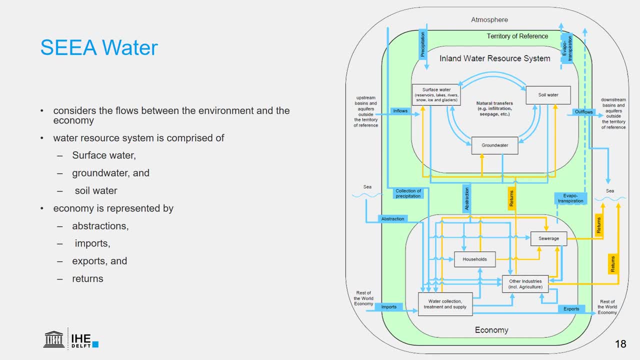 In relation to the economy, it is represented by abstractions, imports, exports and returns of the most relevant economic agents, such as households. the industry involved in the collection, trade, treatment and discharge of sewage. the industry involved in the collection, treatment and. 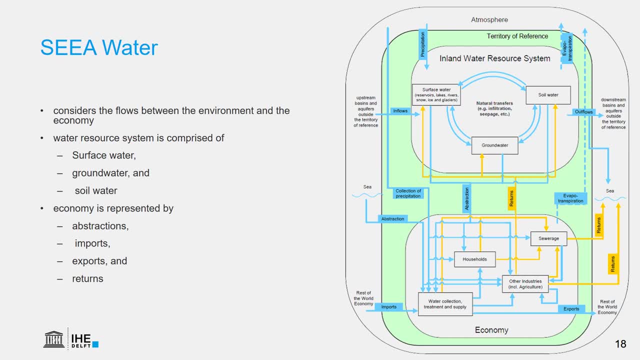 supply of water to households, other industries which use water in the production process and to the rest of the world. The CEA Water Framework has been designed to link the economic information with hydrologic information in order to provide the users with a tool for integrated analysis and, as such, 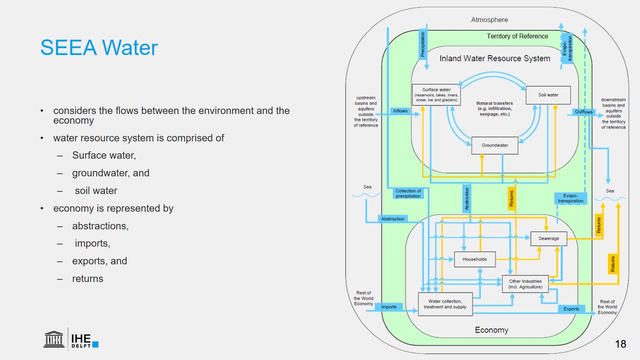 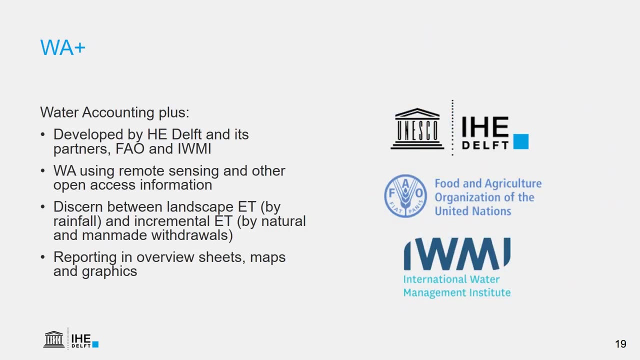 it involves a collection of very detailed data from various sources. To know more about the framework you are referred to, read the CEA Water documentation. Solving water problems requires information from many disciplines and the physical accounts which describe sources and uses of water are the most important foundation. 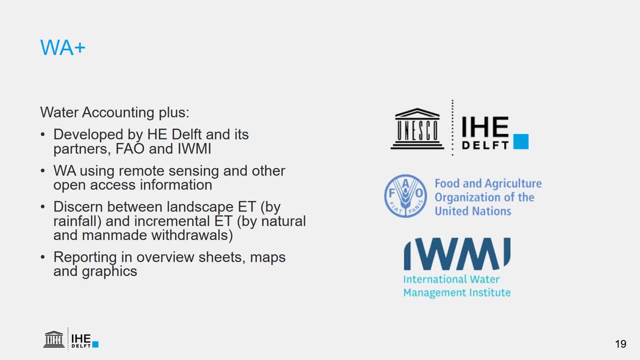 The information has to be coherent and reliable and harmonized in order to provide an integrated picture useful for the assessment of the problems. Water Accounting Plus is a water accounting methodology developed by HE Delft in partnership with IMI and FAO, The geographic domain for Water Accounting Plus. 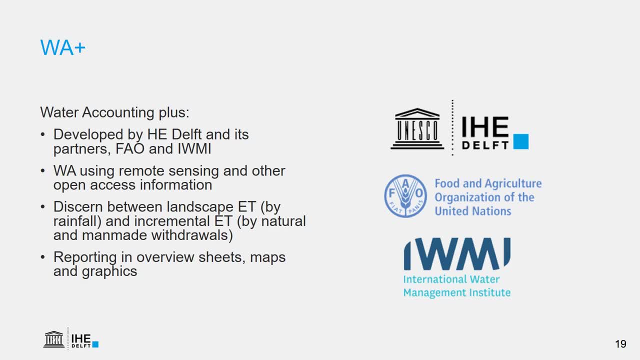 is a river basin And it uses mainly data from remote sensing products and other open access spatial database and information. When data is available, the remote sensing data are validated using ground based observations and literature values. The data collected is then analyzed through standardized analysis method. 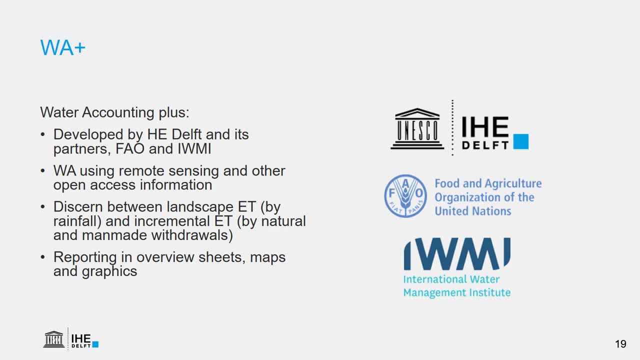 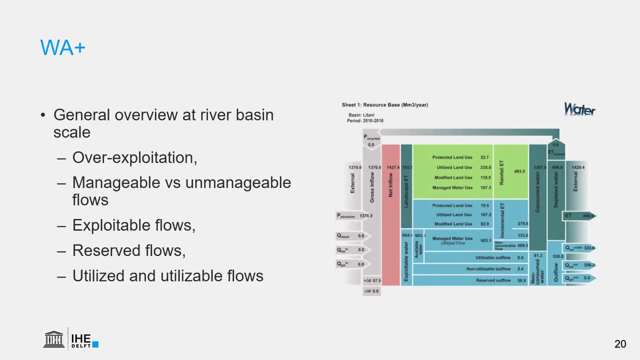 using open access programming tools and scripts, And the results are reported Using standardized overview sheets, maps, tables and graphs. The outputs of Water Accounting Plus provide general overview at river basin scale of over exploitation, manageable versus unmanageable flows, exploitable flows, reserved flows utilized. 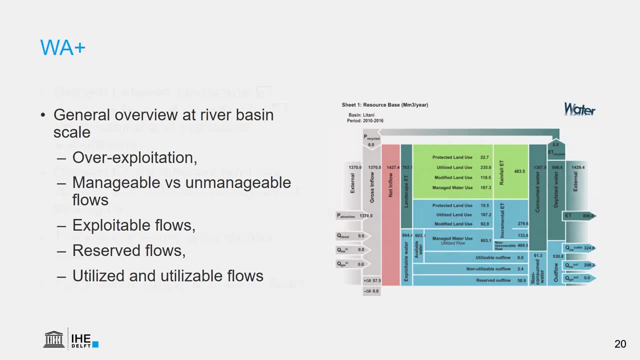 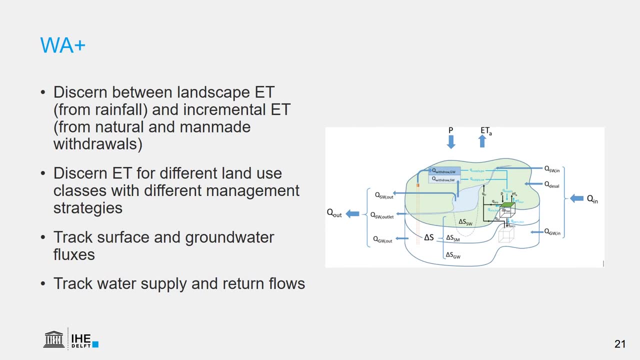 and utilizable flows- Water Accounting Plus. On the link in the description you may find a link to the website for our documented features from the heavenswelung survey. I'd recommend logging back in and studying the main items we talked about before.